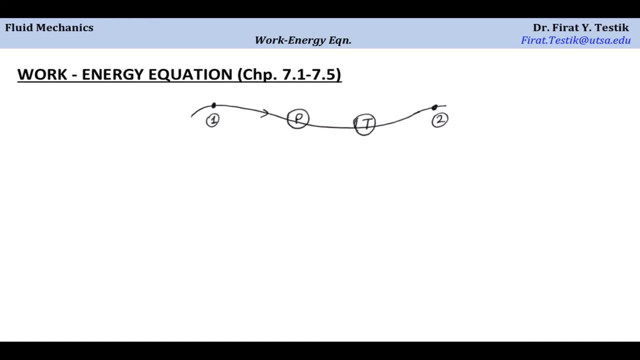 fluid and we may also have a turbine, say, for generating electricity. So if we have such mechanical devices in the flow field, then we need to modify the Bernoulli equation to account for these energy sources and sinks. So remember, in Bernoulli equation we consider two points. when we apply Bernoulli equation and consider that now. 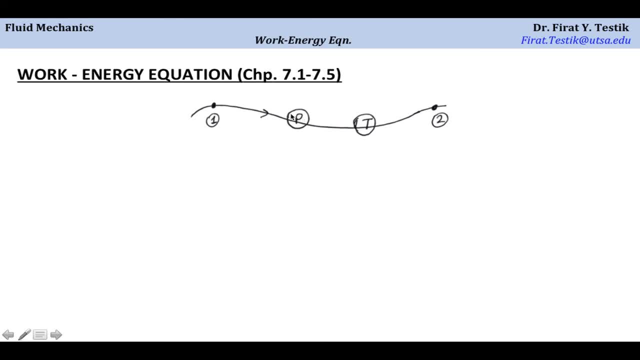 we have two mechanical devices, let's say a pump and a turbine, in between these two points. So if you want to relate the pressure and speed and elevation of point 1 to the pressure, speed and elevation of point 2, now we need to consider the mechanical devices. 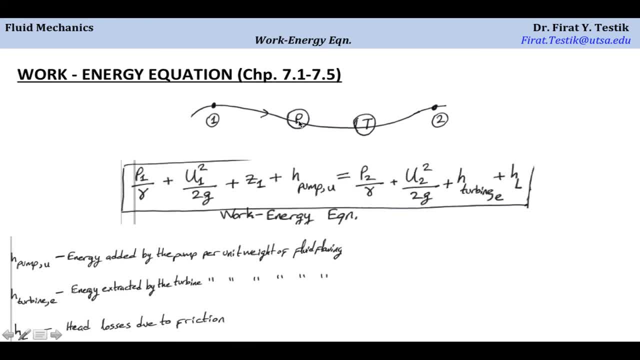 So we modify the Bernoulli equation. remember the first three terms on the left side are the three terms of the Bernoulli equation, left hand side of the Bernoulli equation. So we add this term: h, pump, u and u stands for useful, because pump adds energy. 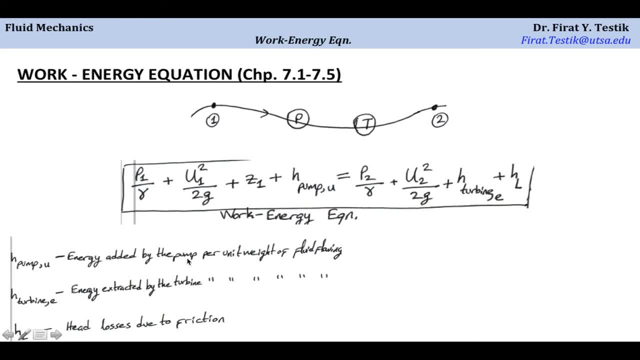 So h pump useful is the energy added by the pump per unit weight of fluid flowing. Then on the right hand side we have these three terms and I noticed that I forgot to put z2 here. There should be a z2 here. please correct in your notes. So this is p2 over Gamma plus u2 square over 2G plus. 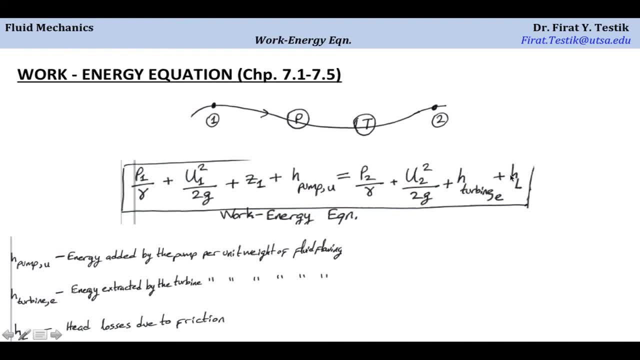 z2, plus H turbine, E, which is extracted, plus HL, which is head loss Now. so these three terms, including the Z term that I forgot to add, are the same terms as the right-hand side of the Bernoulli equation. 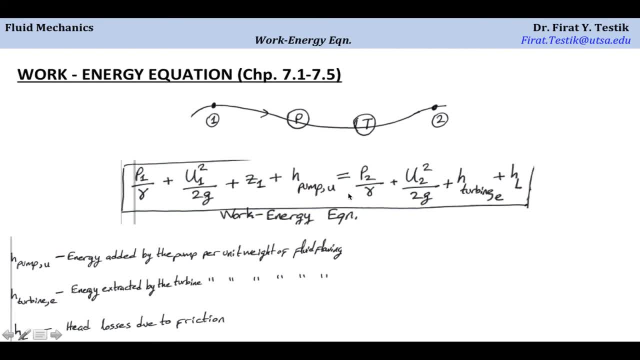 So the new terms that we add for the work energy equation is the H pump, U, which is the energy added by the pump, again per unit weight of fluid flowing. This H turbine E- E is for extracted, because turbine extracts energy from the fluid. 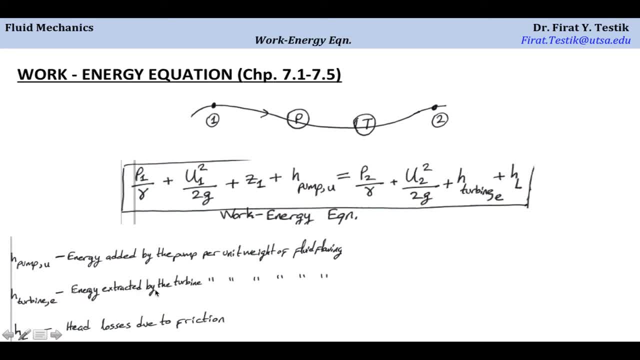 So this H turbine, E stands for energy extracted by the turbine per unit weight of fluid flowing And HL is the head losses due to friction. So let's say, in a pipe we may have friction due to the pipe wall or pipe surfaces and this will introduce head loss. 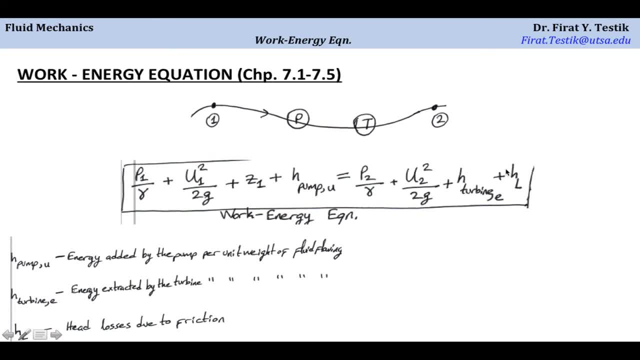 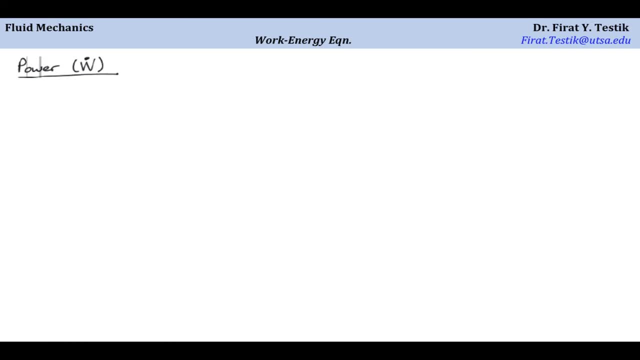 And this term accounts for this head loss. So in engineering equations, in any engineering application, we are typically interested in also the power of, let's say, mechanical devices, such as the power of the engine. So we may have friction due to the pipe wall or pipe surfaces and this will introduce head loss. 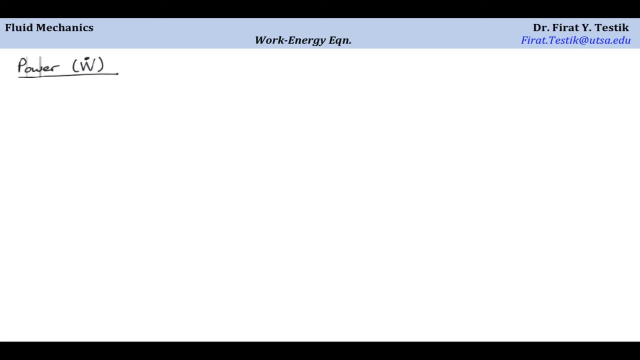 Let's say if we are working with a turbine or pump, we are interested in the pump power or turbine power. So remember that power is defined as energy per unit time And we just considered H pump useful and H turbine extracted. Those are added and extracted energy per unit weight. 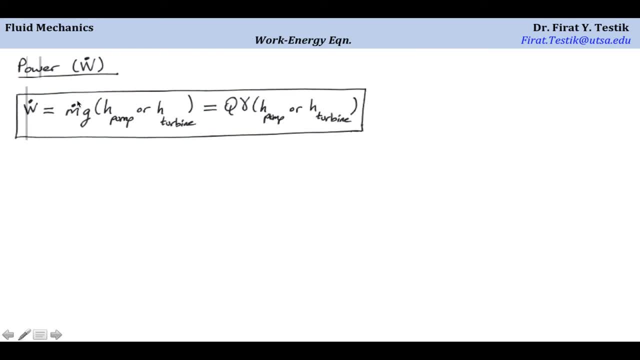 So, if we move on, we multiply this H pump or H turbine, which is energy per unit weight, by weight flow rate, So weight per unit time basically, then we would end up with energy per unit time, which is, by definition, the definition of power. 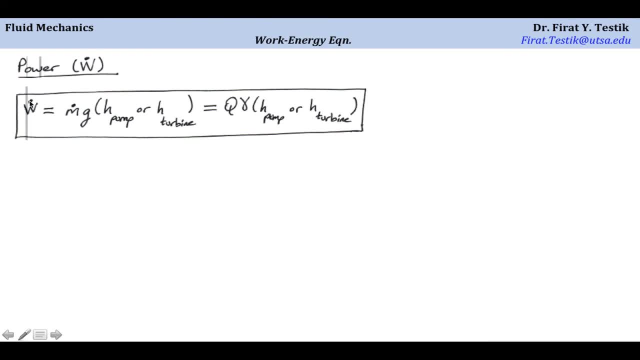 So W dot stands for power In our, in our notation. So power equals to weight flow rate, which is mass flow rate times gravitational acceleration. This would give us weight flow rate multiplied by energy per unit weight. So energy per unit weight multiplied by weight per unit time would give us energy per unit time. 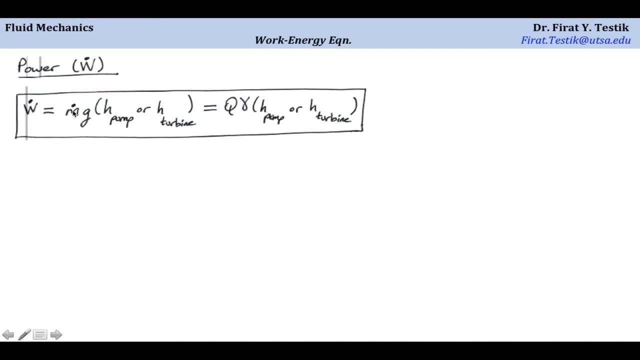 which is power. Now remember mass flow rate. It is also related to volume flow rate through density, rho. So if we write mass flow rate in terms of volume flow rate, which is defined, which we denoted, by capital, Q, So Q times rho, or volume flow rate times density, is mass flow rate. 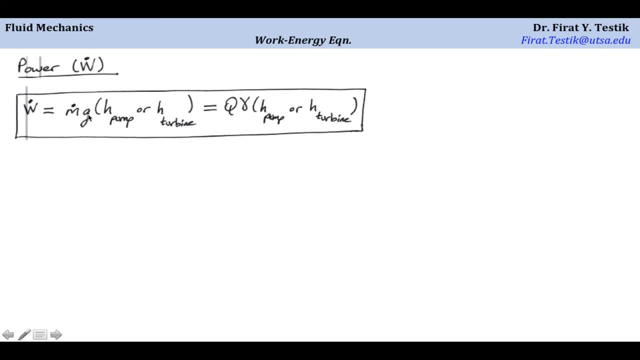 And density times gravitational acceleration. G is specific weight, So we can write weight flow rate as volume flow rate times specific weight, And so our power relationship is volume flow rate times specific weight times H pump or H turbine. Now, as you know, during the conversion process of mechanical energy, 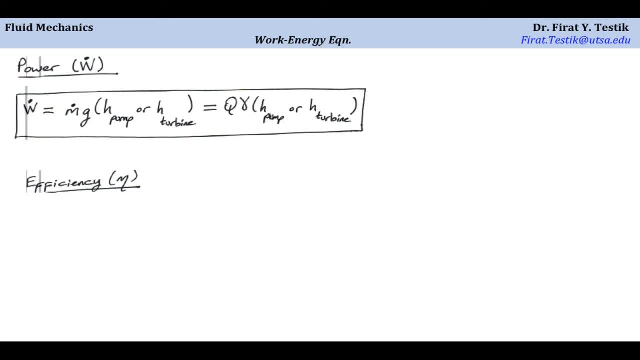 there are losses due to friction. So to quantify the degree of conversion process between the mechanical work supplied or extracted and the mechanical energy of the fluid, we define efficiencies, mechanical efficiencies. So mechanical efficiency for pump. let's say eta denotes for efficiency and eta pump is the mechanical efficiency of the pump. 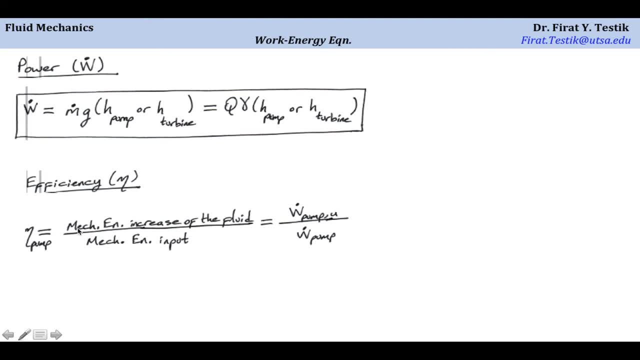 Then it is defined, as you can define it, in terms of either power or in terms of energy. So it is the output power divided by the input power to the system. This is the definition of the efficiency, and efficiency is typically the higher efficiency you have. 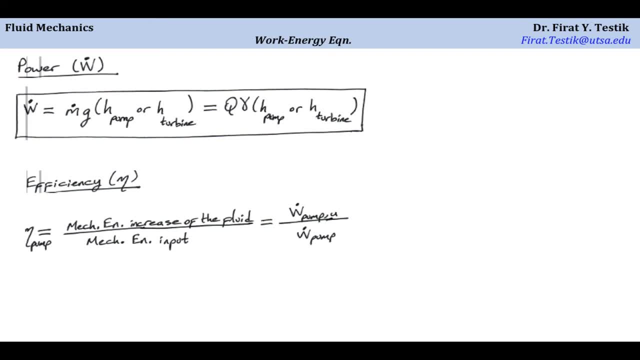 the better the performance of the device. So efficiency uh values varies between zero and one. Okay, So it's important. You cannot have an efficiency larger than one, and zero efficiency means that your device doesn't work. So you can define efficiency as the power output divided by power input. 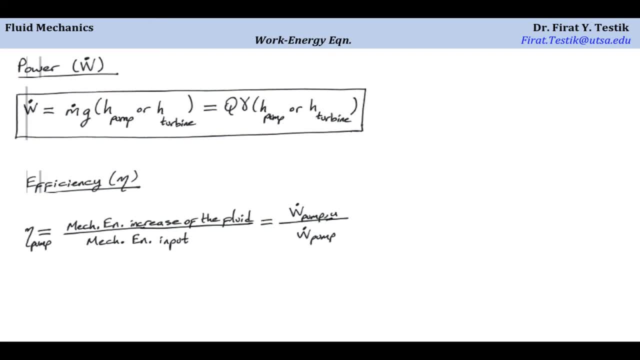 or if the uh process occurs, input and output uh to the system, the system occurs at the same time. Uh remember, uh power is energy per unit time, So we can also define it in terms of energy output divided by the energy input. 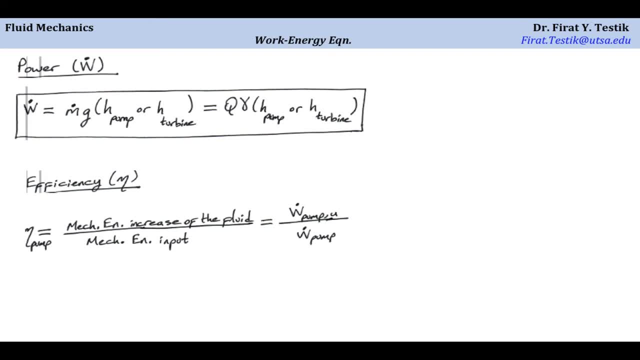 Now for the case of pump. the purpose of the pump is to increase the energy of the fluid. We push the fluid through the pump, So our output is mechanical energy increase of the fluid And our input, our input, is mechanical energy input to the pump. 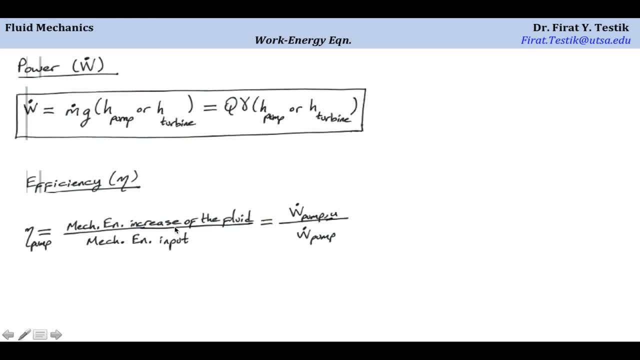 So efficiency of the pump is mechanical energy increase of the fluid divided by mechanical energy input to the pump. or we can write it in terms of power as well. So we can write it as the useful power of pump divided by input to the pump: power input to the pump. 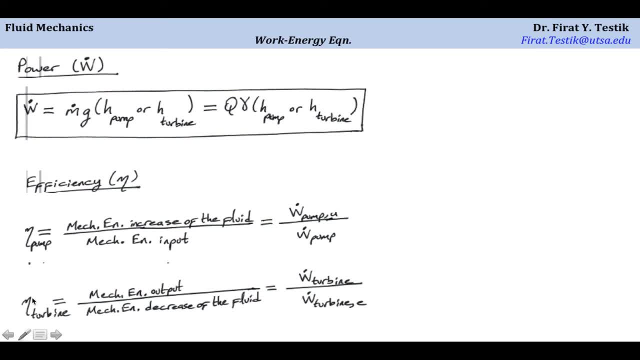 And for the turbine case, we can write the mechanical efficiency of the turbine as the mechanical energy output from the turbine divided by mechanical energy decrease of the fluid. Remember, turbine extracts energy from the fluid and uh converse it to a rot. Let's say if it is a rotational. 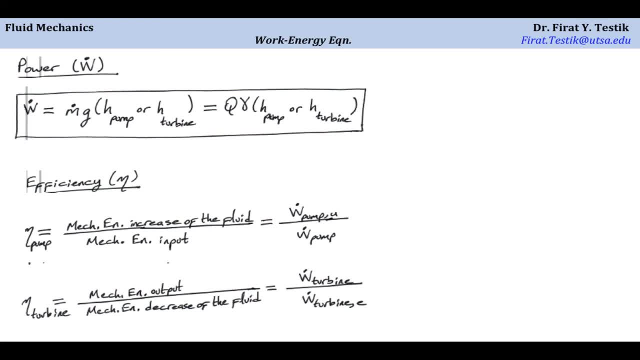 then uh, it creates a rotational uh movement. So the input to the turbine is mechanical energy: uh decrease of the fluid. So we can also write this in terms of power: power of turbine, uh output divided by 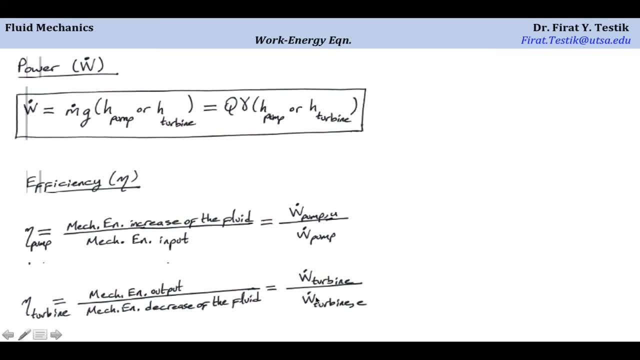 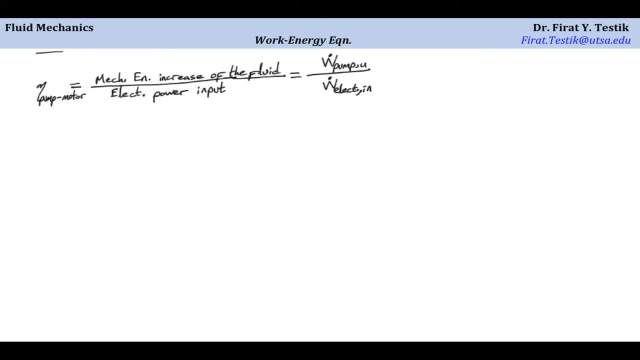 uh power extracted by the turbine Now typically uh pump uh and turbines uh do not appear uh in a uh flow system. Uh, we typically have an assembly of pump and motor and a turbine and generator. 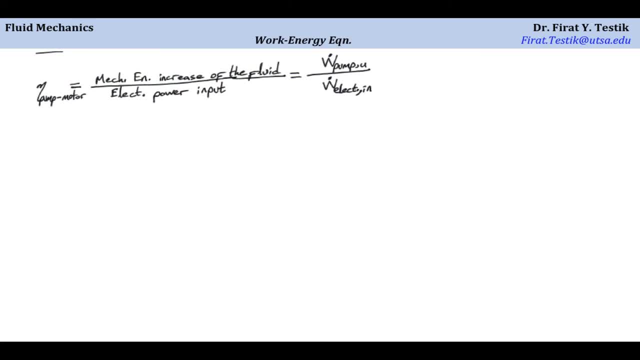 So motor provides the mechanical motion uh input to the pump, which then increase the uh energy of the uh fluid. and for the turbine case we typically use a generator. turbine generates a mechanical motion and the generator takes this mechanical motion and 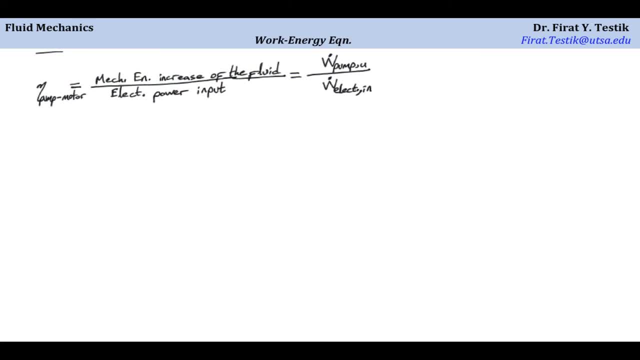 converts it into electricity. so if we have a pump and motor system, the input, the output of the system is mechanical energy increase of the fluid, because pump pushes the fluid, and input to the system is input to the motor, which is electrical power input because by definition, motor takes electrical 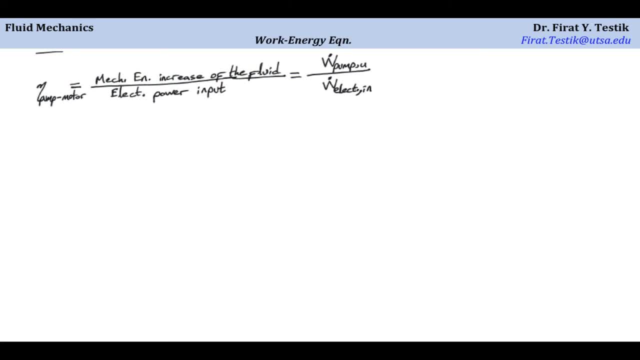 energy and then converts it into mechanical energy. so we can write the efficiency of the pump and motor system as the power- useful power by the pump divided by the input, electrical power into the system for the turbocharger turbine generator. the turbine and generator assembly provides electricity, electrical power. so our output is: 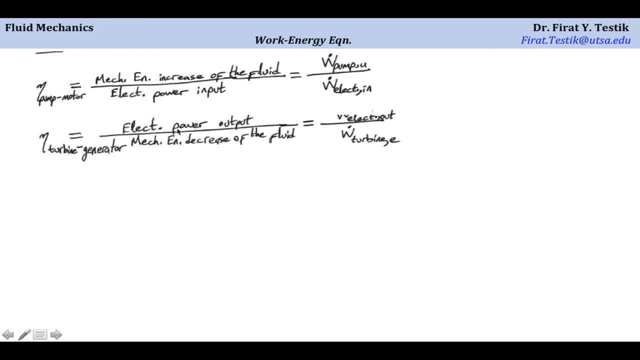 electrical power output divided by, or electrical energy. this should be energy. now we are talking about energy divide by energy, so this should be electrical energy output divided by mechanical energy: decrease of the fluid, because input is the fluid. energy to quadr: awf, w1, e2, e3. 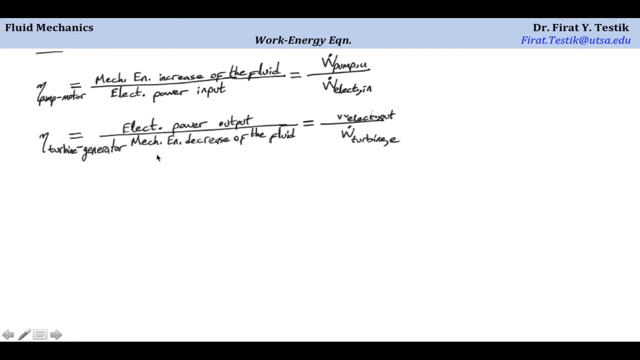 e4, e5, e7, c, d power by the turbine. now I would like to talk also another important concept. this is kinetic energy correction factor. we will denote kinetic energy correction factor by alpha. you can see here now. remember we talked about, let's say, in a 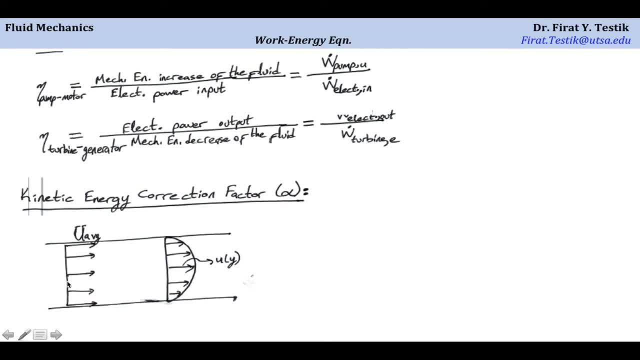 pipe flow. we may have a uniform flow velocity profile, as you can see here, and if we have a uniform velocity profile we can represent the speed as, let's say, speed average. this is you average. all of the speed values are identical. it's a uniform profile, but in general, typically we have non uniform velocity profiles. 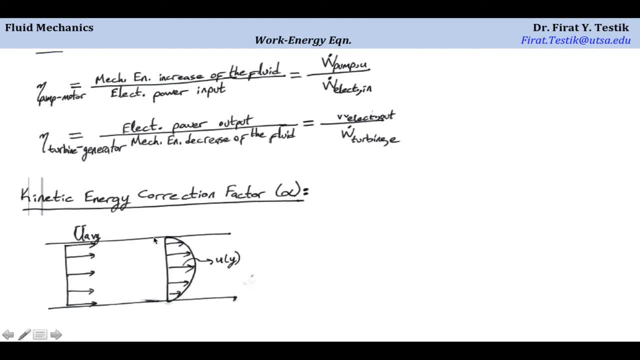 such as this one, this parabola, because there is friction on the wall and these friction will create no slip boundary condition at the wall. so we would observe such non uniform velocity profile and remember we define volume flow rate as the area cross-sectional area. if this is pipe, it's the cross-sectional area of 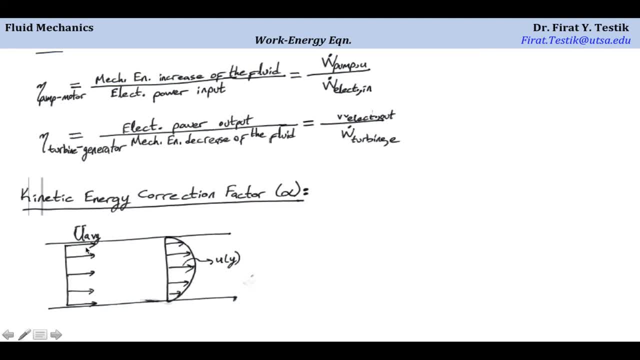 the pipe multiplied by this average speed, if we have a uniform, uniform Velocity profile. but if we don't have a uniform velocity profile, remember, we use differential volume flow rates and We consider all of these differential volume flow rates at different, You know, across this cross-sectional area, and then we integrate. 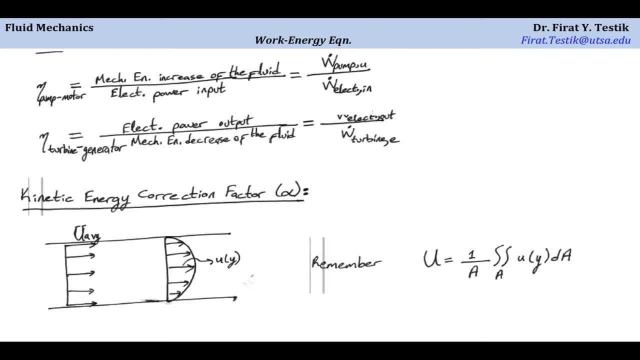 Volume flow rates, these differential volume flow rates, through these differential areas, to obtain the Total volume flow rate in this or through this cross-sectional area. then Remember, we defined U, capital U or the average U as the Fictitious of speed which is defined, which would give you the same volume flow rate as 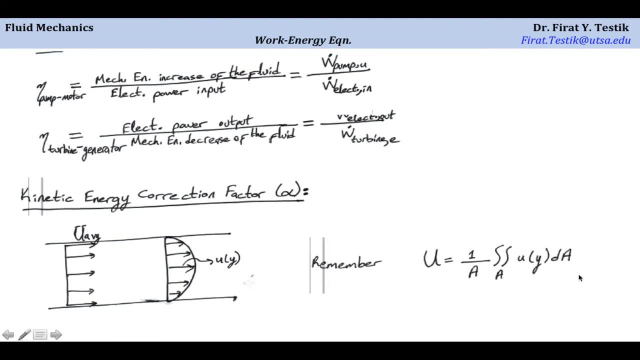 the individual. you know differential volume flow rates integrated. so basically We need to calculate the volume flow rate through these individual differential volume flow rates through differential areas, and then calculate the total volume flow rate through integration and if you want to define a fictitious speed That would give us the same volume flow rate. 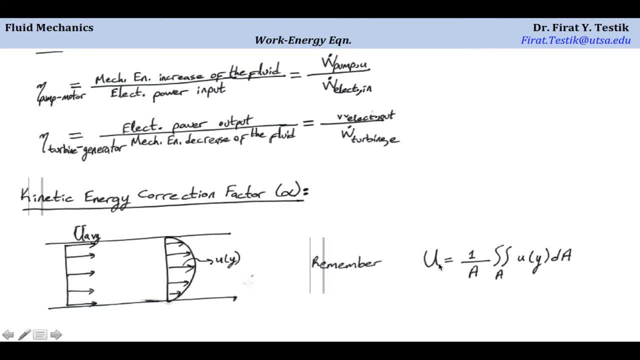 So we need to equate them, which is basically: u times a would be equal to aerial integral u, y, da. and Remember this is how we defined the average speed: fictitious average speed, as u equals to 1 over area, cross-sectional area multiplied by the aerial integral of. 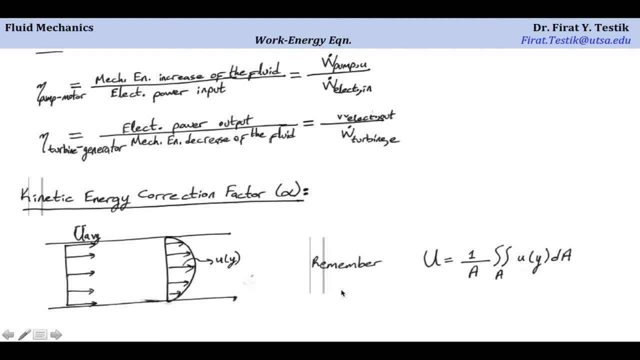 Uy da, this you. this is the speed at different Locations and Da is the differential area. so u y da would give you differential volume flow rate. Integration of it would give you the total volume flow rate divided by the area, would give you the fictitious average speed. 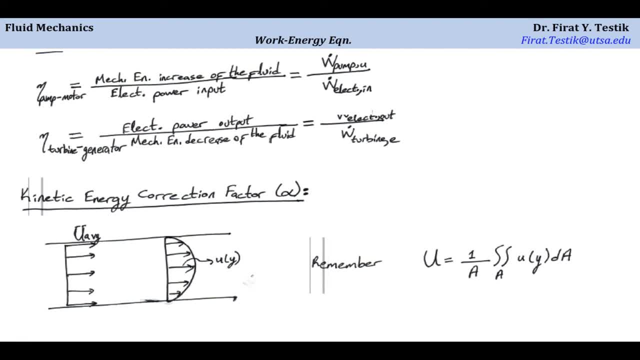 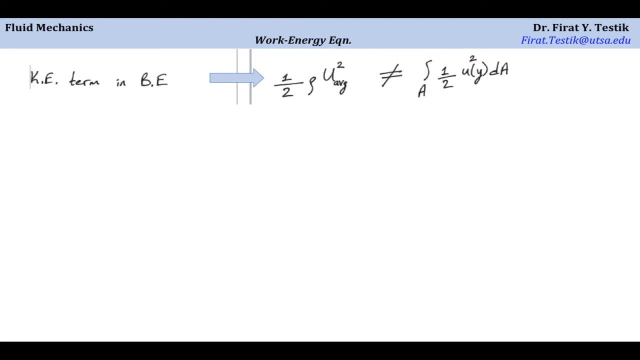 This is what we did For when we were discussing about, Let's say, flow rates When we have non-uniform speed. now, The kinetic energy term in Bernoulli equation- Let's focus on that- It is one half rho u average square. This is after manipulation, It's the same. 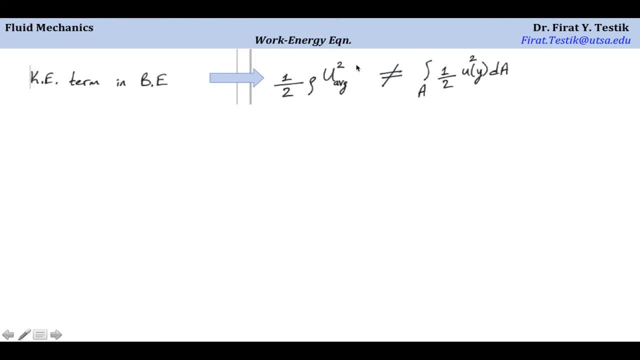 Basically term. so this is the kinetic energy term in the Bernoulli equation, or the second term in the Bernoulli equation, on the left side or right side, doesn't matter. second term. so this: in this in the Bernoulli equation and also in work-energy equation, we consider speed square and 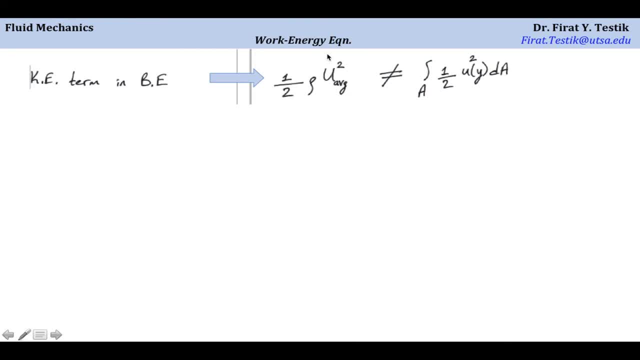 This is the average speed that we consider. If we have a uniform velocity profile, this is perfectly fine, but typically we may not have a Uniform velocity profile. if we have a non-uniform velocity profile, then we need to consider the differential kinetic energies, as here, and then we need to integrate throughout the cross-section. 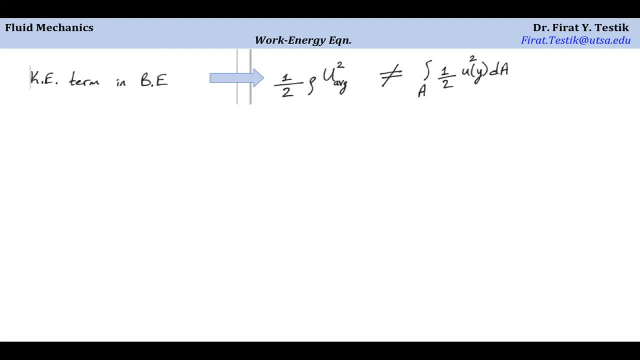 or over the cross-sectional area. Now, mathematically these two expressions are not identical. So so far we considered this is how we should be calculating, where we considered, if we have uniform velocity profile, we could replace this term in the kinetic in the Bernoulli. 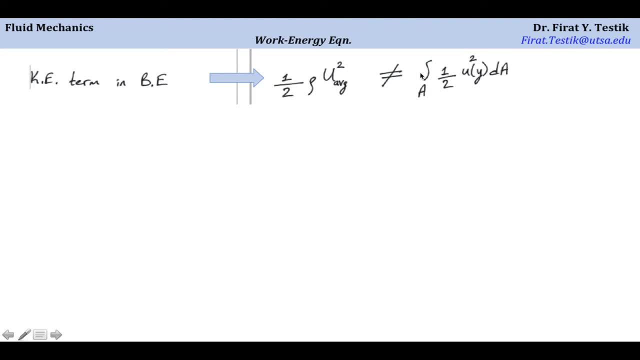 equation and also work energy equation. we replace this term using this term, defined in terms of the average speed. This is fine if the flow velocity is uniform or flow profile is uniform, But, as I said, the flow speed, flow profile, speed velocity profile may not. 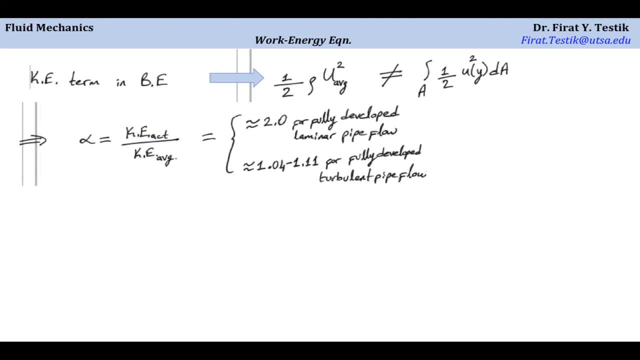 be uniform And in that case we need to introduce a correction for the this inequality. So we define alpha as the kinetic energy correction factor and it is defined as the actual kinetic energy divided by the average kinetic energy. So average kinetic energy is this term and actual. 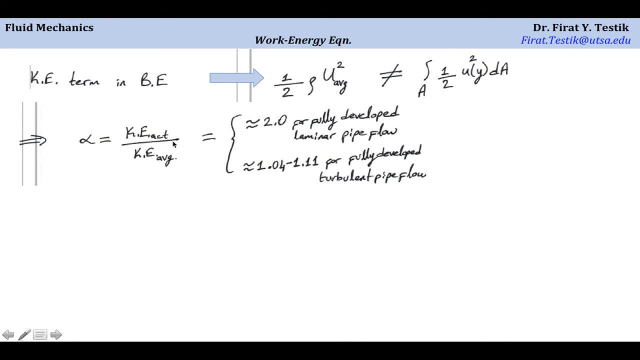 kinetic energy is this term, So we can write actual kinetic energy as alpha times, average kinetic energy. And if we know this alpha value then we can correct our Bernoulli equation calculations and also work energy equation calculations. Now for fully developed pipe flows, the correction factor alpha is approximately equal to 2 for 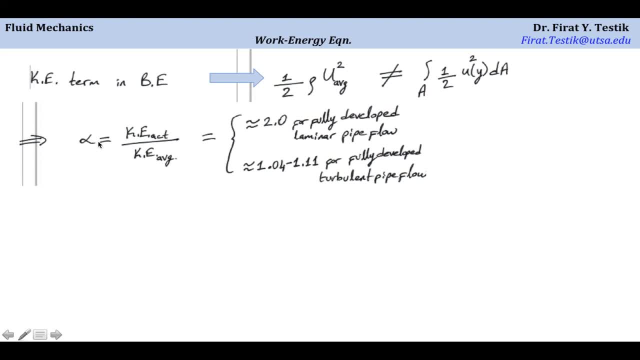 laminar pipe flows And the value of alpha is approximately equal to 1.04 to 1.11.. So there is this small range of values between 1.04 to 1.11.. This is for turbulent pipe flows. 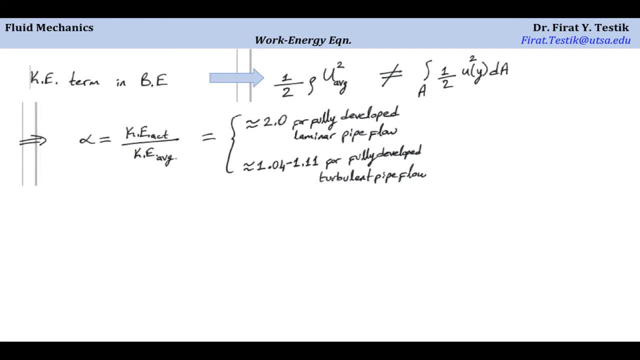 We will soon discuss what laminar pipe flows and what turbulent pipe flows are, But for now just know that these are two different types of turbulent pipe flows. These are two different flow regimes. So if we have laminar pipe flows, we would use 2, and if 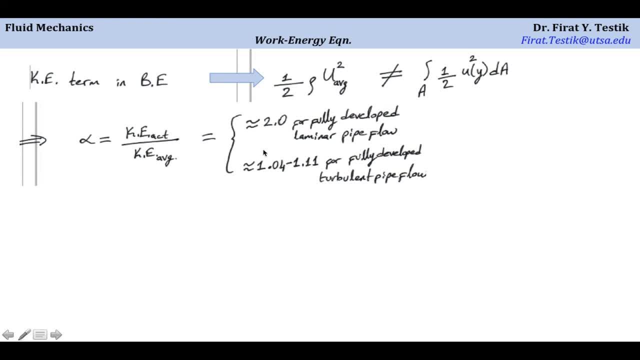 we have turbulent pipe flows, we would use the value given, which is going to be within this range of values. So we can correct Bernoulli equation by introducing a kinetic energy correction factor, alpha 1, in the second term here and another correction factor here in the second term on the right hand side. 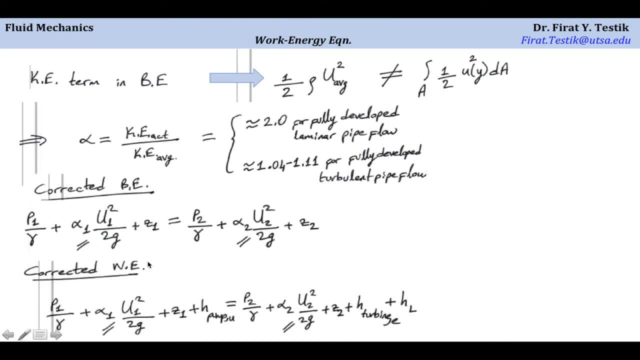 as well. And we can also correct the work energy equation by introducing this alpha 1 in the second term of the left-hand side of the work energy equation and alpha 2 in the second term of the work energy equation on the right hand side of the equation. So now, if 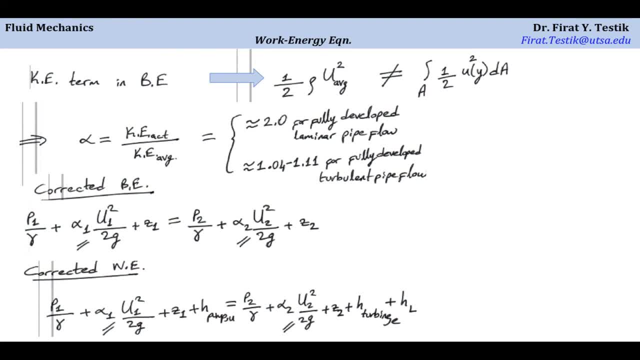 the flow problem specifies an alpha value, then you need to use this alpha value to calculate bernoulli equation or work energy equation. if it does not specify, you can assume that alpha equals to one and alpha equals to one basically assumes that velocity profile is uniform and that's how. 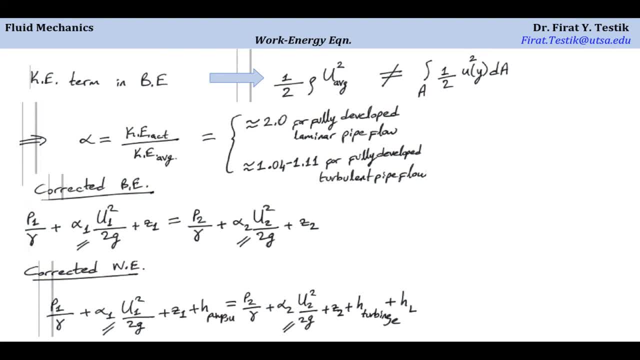 we were solving now. one good thing is: alpha equals to 2 would make significant changes in the values here. however, you will learn that laminar pipe flows are slow flows. laminar, laminar flows are typically slow flows, so this term u square over 2 g, is not very large. 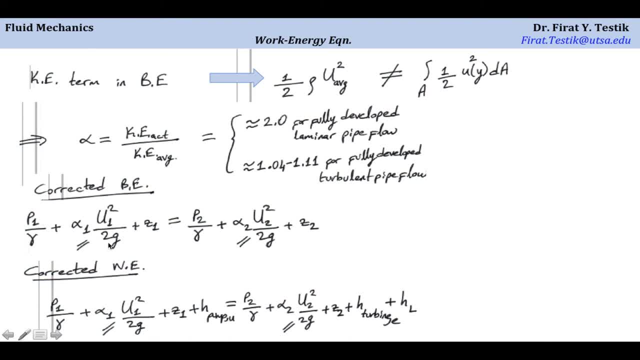 compared to the other terms. so multiplying this term with one or two does not change the result much so. sometimes we neglect- although we know that it is laminar pipe flow- we may neglect this kinetic energy correction factor. now for turbulent pipe flows. the flow velocities are typically fast or 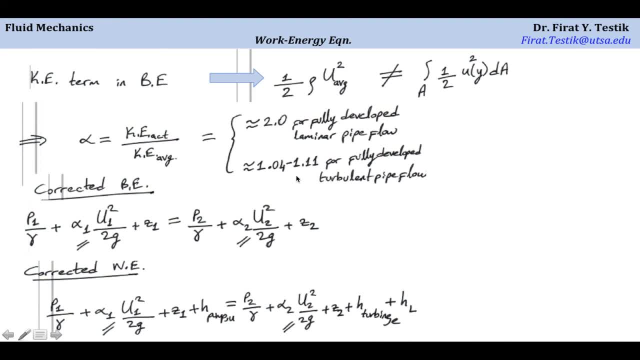 large, and if flow velocities are large, the second term is also large. so it is important with respect to the other terms in the equation. however, now, kinetic energy correction factor, as you can see, is rather small. it's almost or is close to one. so the introducing or the implementation of the kinetic energy correction factor, 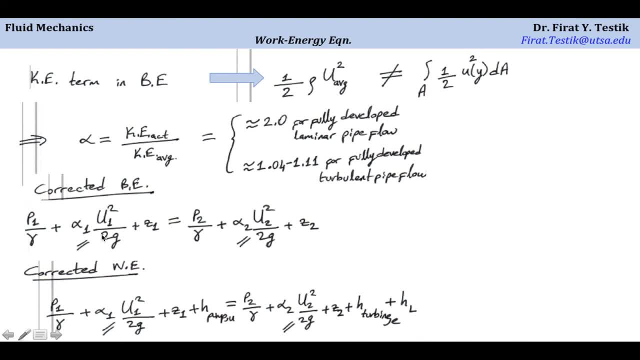 will not change the result much for most of the time. so that's why we may just simply neglect the actual alpha value. we may use one unless it is specified in the given problem. but if it is given in the problem, then we need to use the actual alpha value for that problem. 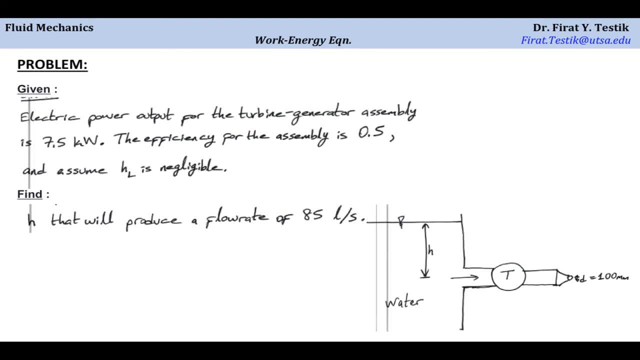 now let's solve an example problem to demonstrate the work energy application of the work energy equation. now let's consider that we are trying to. we want to generate electricity using a turbine generator assembly. here we have a turbine generator assembly and we want to have an electrical power output of 7.5 kilovolts. we know the turbine. 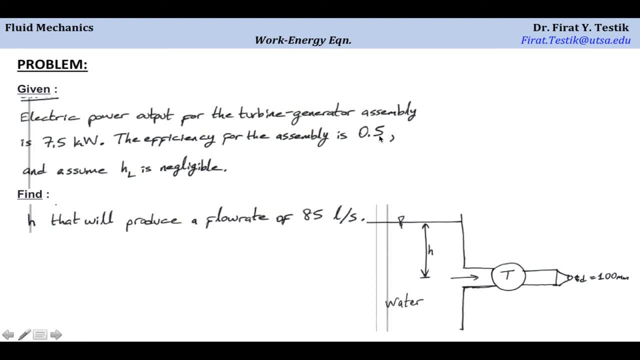 generator assembly efficiency is 0.5. it's given in the problem and we will neglect the head loss in this problem. so basically we are going to neglect the frictional effects. so in this problem we are asked to find h, which is the vertical distance between the free surface. 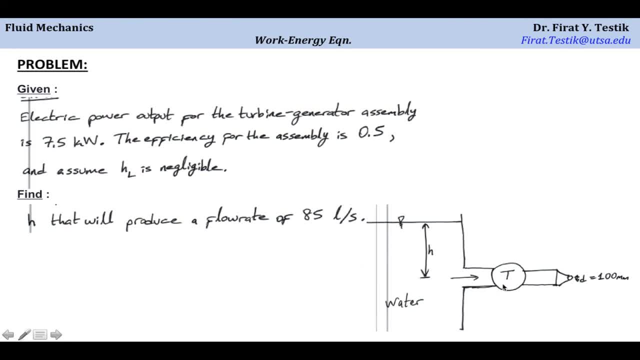 to the pipe generator assembly and our goal is to produce 85 flow rate of 85 liter per second. okay, so we will. we want 85 liter per second flowing through this turbine generator assembly. so what would the value of h be for that 85 liter per second flow rate? also in the problem schematic. 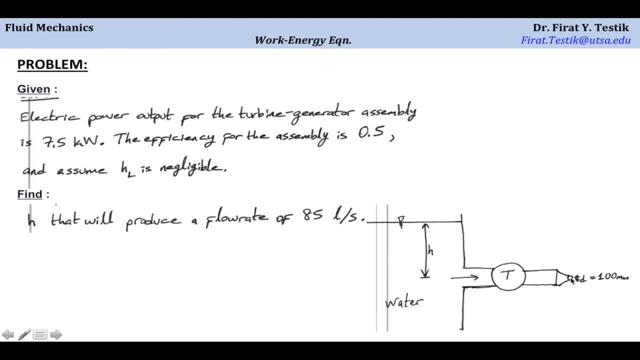 you can see that diameter of the nozzle or outlet is given as 100 millimeter. so here i would recommend that you stop the or pause the video and try to solve this problem on your own, and then start the video and compare your solution with the solution that we will discuss. 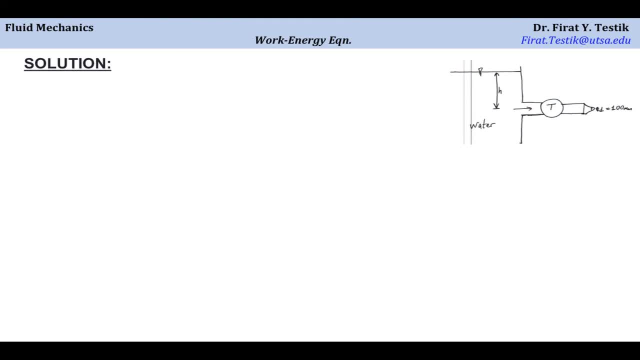 so here i include the schematic on the right hand side so that you can remember the problem schematic. so we will apply work energy equation for this problem and similar to bernoulli equation for work energy equation, we pick two points so that we can write the work energy equation between these two points in this problem we will pick point one as the water. 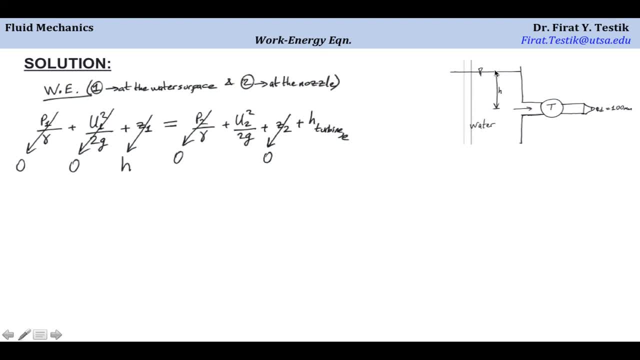 surface, because at the water surface this point is exposed to atmospheric conditions and we know the pressure on the water surface below. in this case your weight at the water surface is less. so in this case you open this problem, as in this problem, and you get also the Integral Tusions. 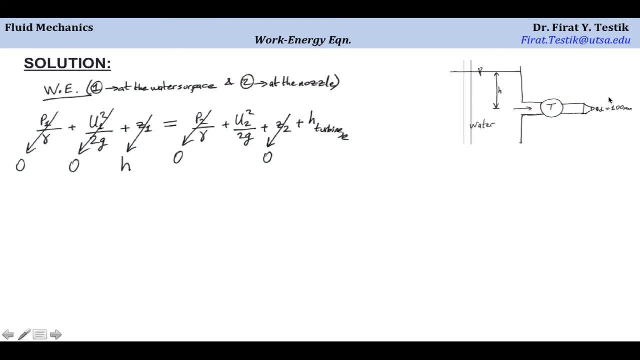 for thesevant Whitney tones like this. and again you see the power energy equation to reduce the unknowns. So if we write the work energy equation between points 1 and 2, we will have p1 pressure 1 over gamma plus u1, square over 2g gravitational acceleration plus z1, which is the elevation of point 1. 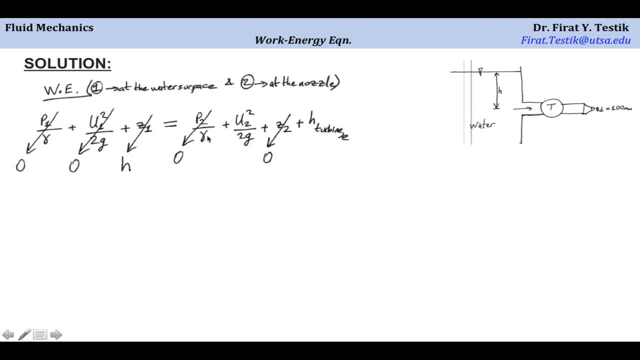 equals to p2 over gamma specific weight plus u2 squared speed at 2 square, divided by 2 times gravitational acceleration plus z2, which is the elevation at point 2 and the H turbine extracted. So this is the energy of the flow extracted by the turbine. Now we know that point 1 is exposed to. 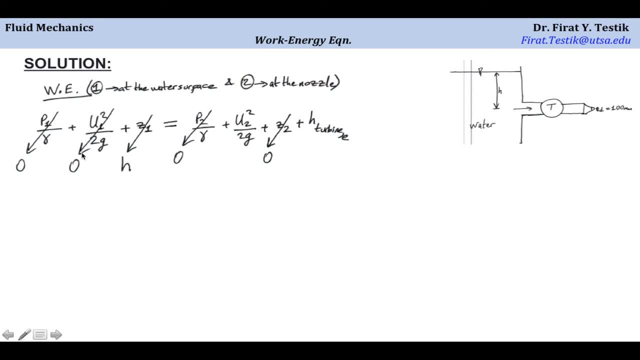 atmospheric condition is exposed to. atmospheric condition is exposed to atmospheric condition. if we work with gauge pressure, then pressure is equal to 0 at 0.1, and same thing for 0.2 pressure at 2: it is equal to 0. we are generating electricity in a. 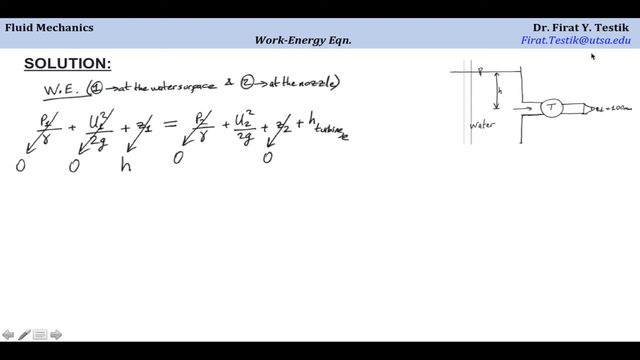 large reservoir, so the speed at 0.1 is not large, because the you would typically not see much of a change in the free surface in a reservoir or in a lake when you generate electricity. right, it's a very large reservoir so you want, we can assume that it's approximately 0. now, if we consider our datum is at 0.2. 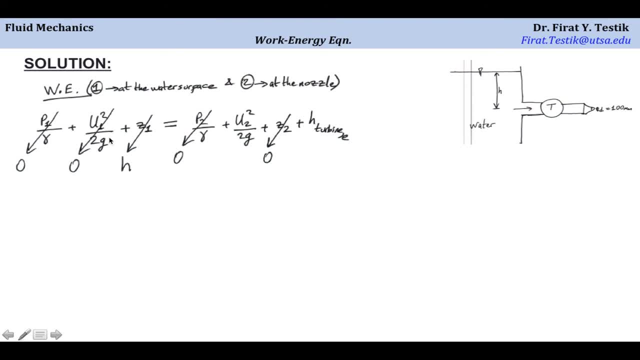 here. then Z1 would have an elevation of H and Z2 would be equal to 0, because this is where our datum is. so we would obtain that H equals to U2 square speed at 0.2 square, divided by 2 times gravitational acceleration, plus the 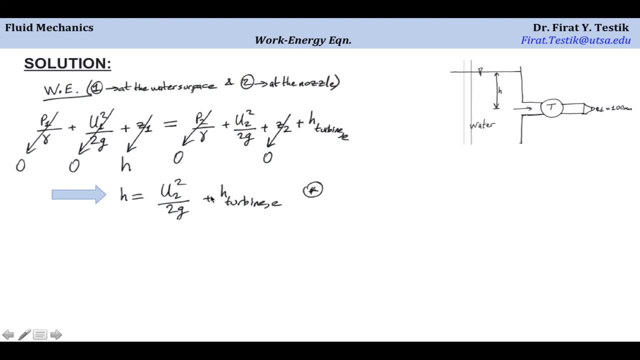 extracted flow energy by the turbine H, turbine E. so to be able to solve the value of H, which is the unknown quantity in the problem, we need to find U2 and also we need to find H turbine extracted. now U2 is pretty straightforward in the problem. volume flow rate is given Q2. 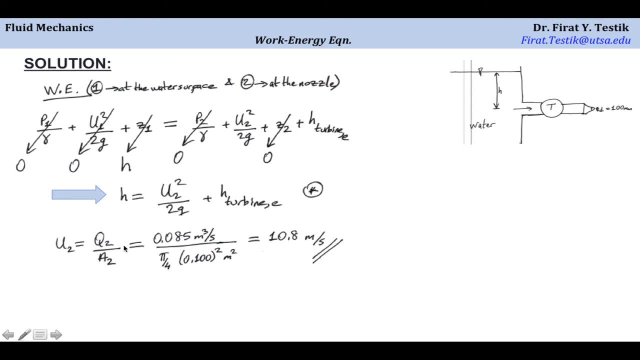 is given. we can easily calculate a2 because we know the diameter here given as hundred millimeter at the outlet. Q2 is given in terms of eighty-five liter per second, and 85 liter per second equals to 0.085 meter cube per second. remember the. 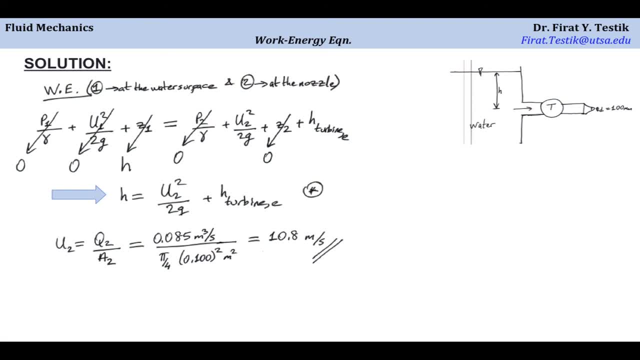 conversion between liter and meter cube is one. meter cube is thousand liters, so if you do the conversion, then volume flow rate at two is 0.085 meter cube per second. divided by area this is a circular area, so it is pi over 4 times diameter square. now it is 100 millimeter. so the diameter 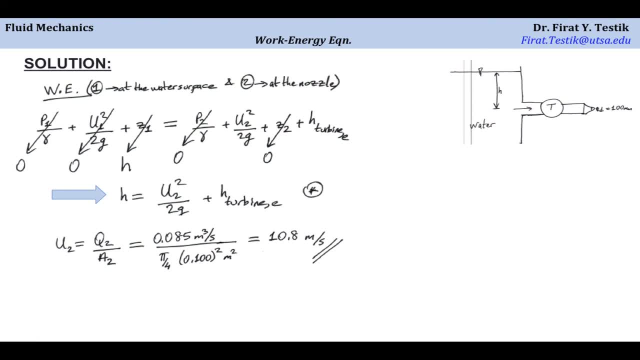 is 0.1 meter. so if you do the calculation you can show that u2 is 10.8 meter per second. we know g, which is gravitational acceleration, which is it is 9.81 meter per second square. so we know this first term. now we need to find h turbine e. 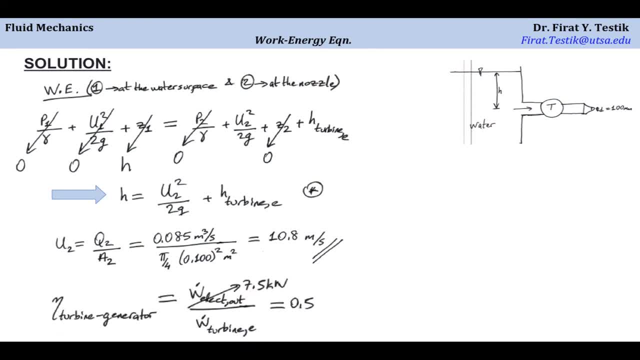 now for this purpose. we know that turbine generator assembly has an efficiency of 0.5 and also in the problem, the it's given that the turbine generator assembly produces a power output of 7.5 kilowatt. remember, efficiency of turbine generator assembly is defined as output. 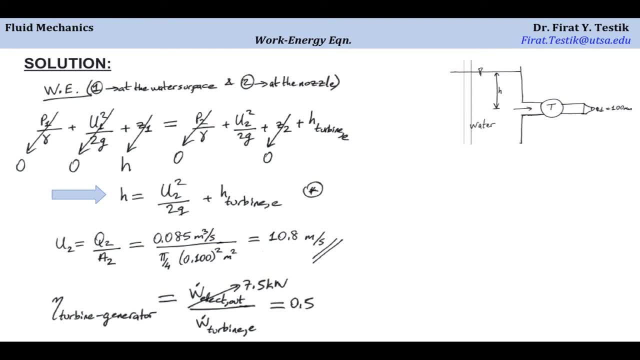 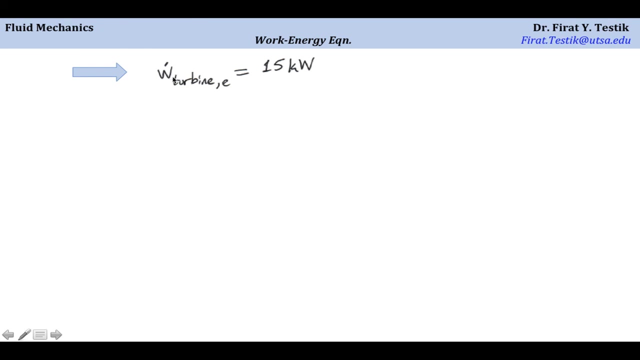 which is given in the problem is 7.5 kilowatt divided by the input power to the assembly, which is the extracted power from the flow by the turbine, which is shown in the denominator here, and it's equal to 0.5. so you can calculate the power of extracted power by the turbine as 15. 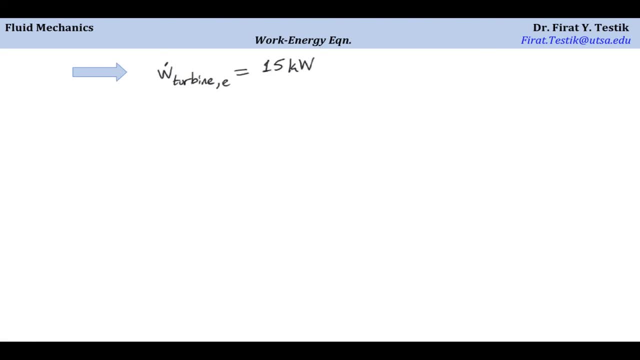 kilowatts and remember the definition of power as 15 kilowatts right from a turbine generator. studying is a structure and so it should. quis establish theve power from the flow here for challenge. so we have the eliminator here, and fw, which also means the electric currentえて, as doubleavala circuit this motorаков Она. 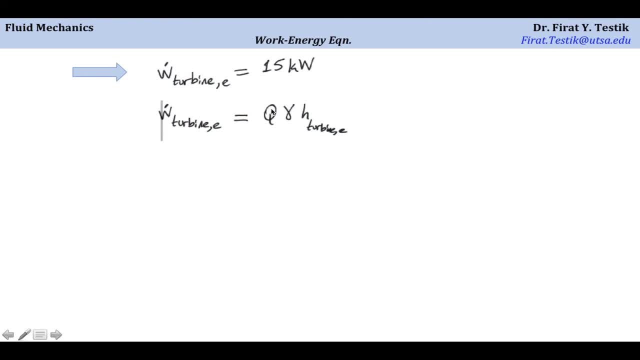 power. power is defined as volume flow rate times, specific weight, which is weight flow rate right. this combination, multiplied by H turbine extracted and H turbine extracted, is the quantity that we want to calculate so that we can plug it into the work energy equation to solve the problem. now, in this problem we 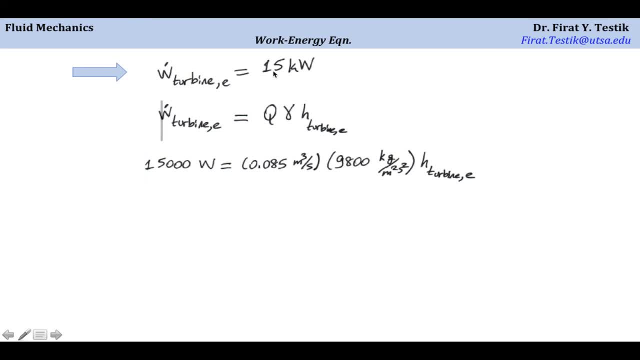 know the, you know, so far we have calculated the extracted power: 15 kilowatt, so we can write it as 50,000 watts, and it is equal to volume flow rate, which is 0.085 meter cube per second, times specific weight, which is density of water, times gravitational acceleration, which is 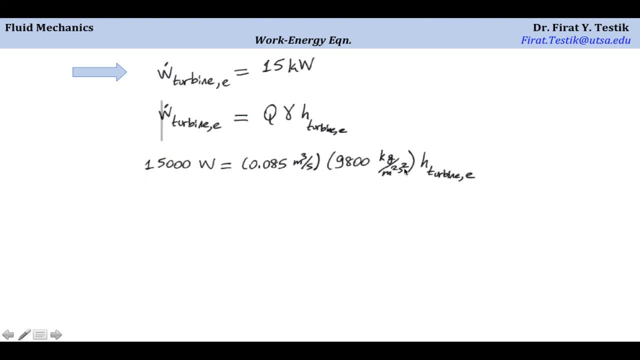 ninety eight hundred kilogram per meter squared squares per second square. this is specific weight of water and H turbine extracted is what we want to calculate from this power equation. so if you do the calculations you can show that the extracted flow energy by the turbine is per unit weight is 18 meter, so we can plug this value into equation star, which. 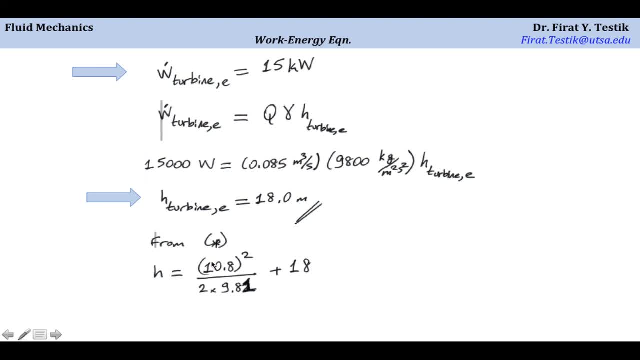 is a the work energy equation. we know that speed at point two we just calculated as 10.8 meter per second. so we take the square divided by two times gravitational acceleration, plus H turbine E, which is 18, so you can show that the H, the